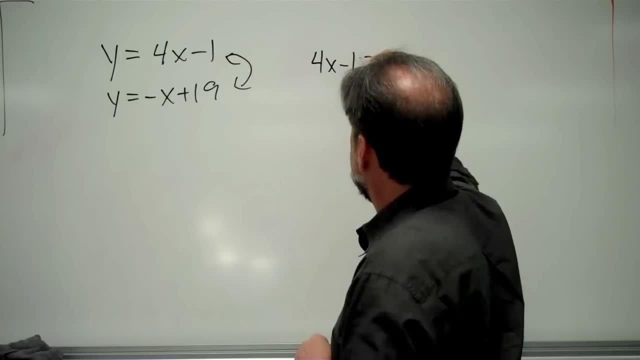 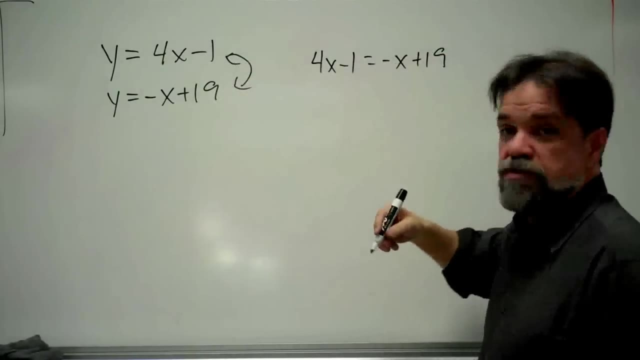 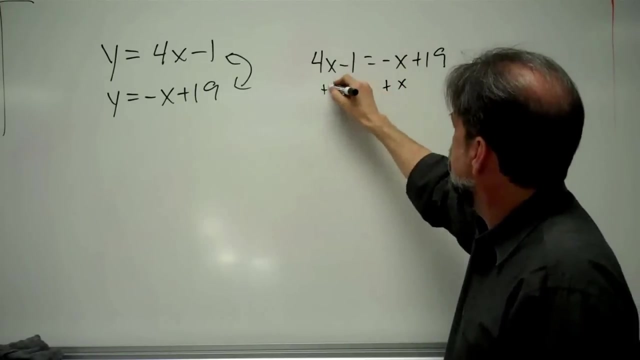 So what we do is We set up: 4x minus 1 equals negative x plus 19.. Have one equation equal the other equation and just solve that Not so hard. A lot of x's up there. Let me add x to this side. 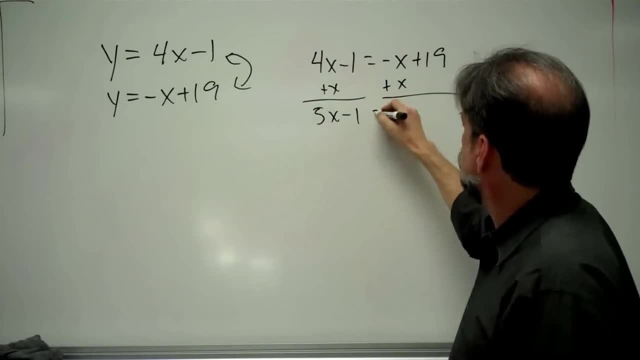 Add x to this side And now I've got 5x minus 1 equals 19.. I'm going to add 1 to both sides here And I get 5 times x equals 20. Which means x must equal 4.. 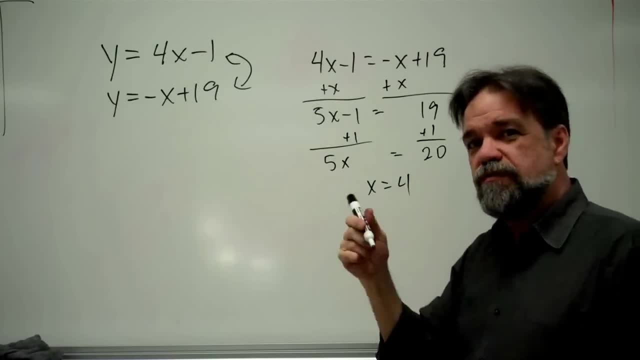 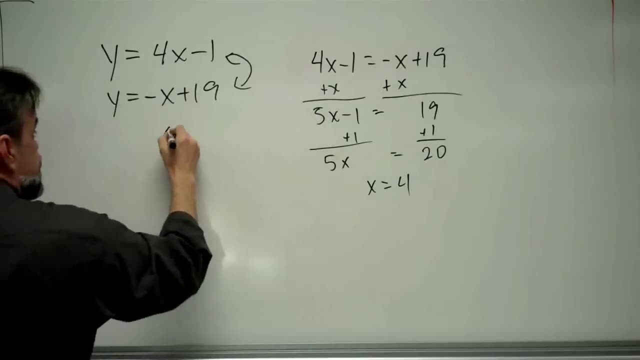 Great, OK, Am I done? No, I'm looking for a point and all I have is an x. I still need a y-coordinate. OK, So it's going to be 4.. Oops, It's going to be 4 something. 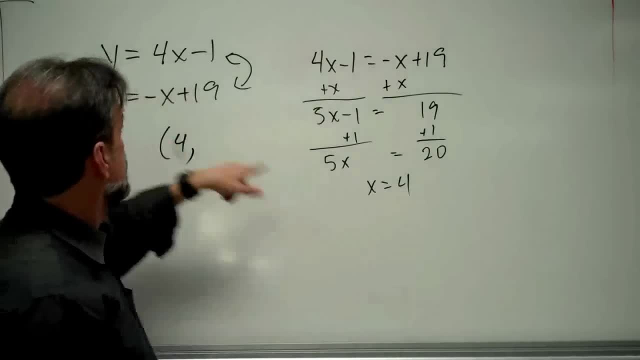 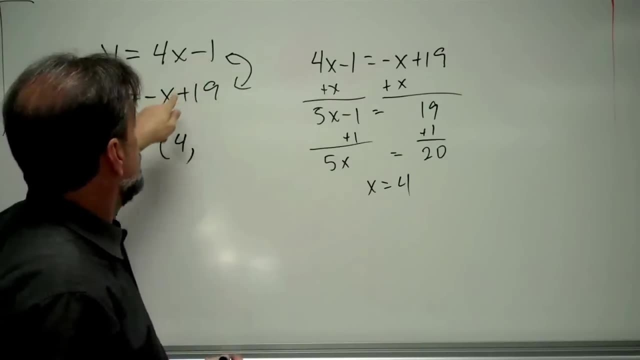 How do I find the y-coordinate? I take my 4 and I plug it right into Either one of the equations. My preference is both equations, Because if you can put it into both equations to get the same y-coordinate, You know you're right. 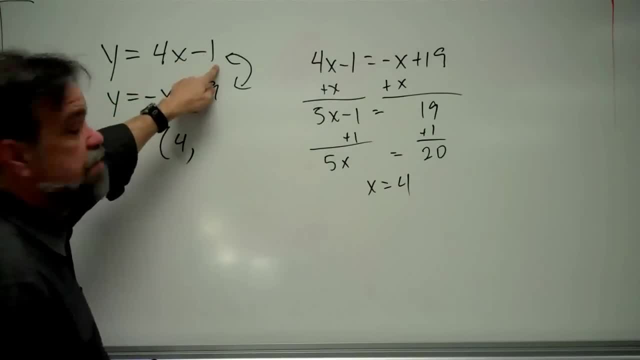 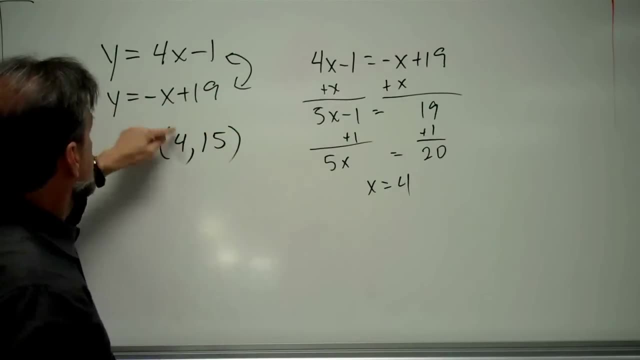 Okay, So 4 times 4 is 16 minus 1 is 15.. So that must mean our answer is the point 4, 15.. Maybe Let's see Negative: 4 plus 19 is also 15.. So yes, now I know, it's exactly right. 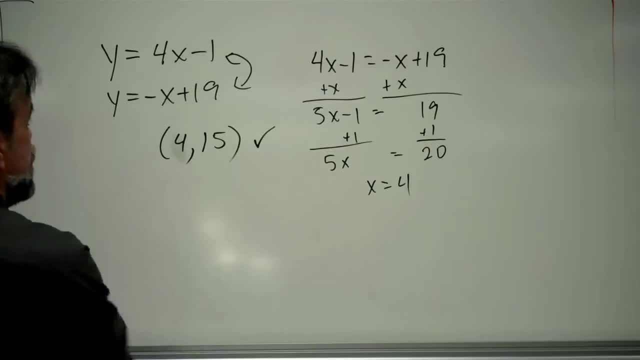 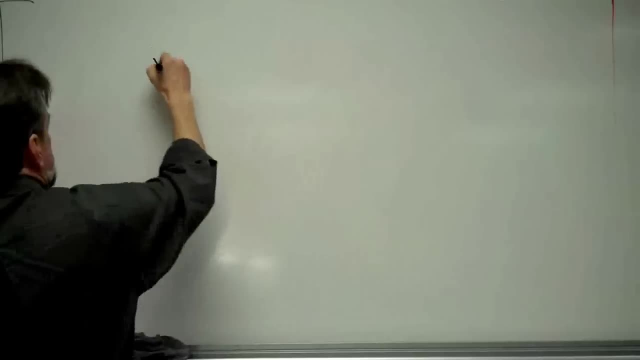 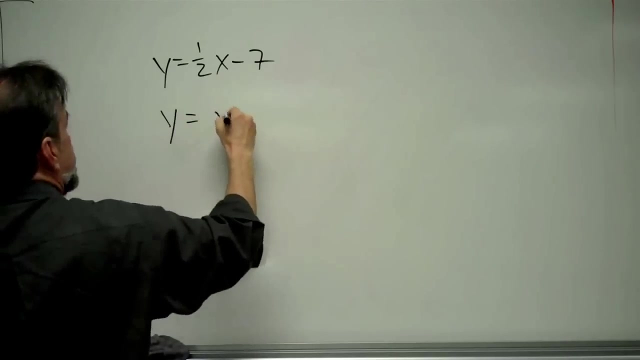 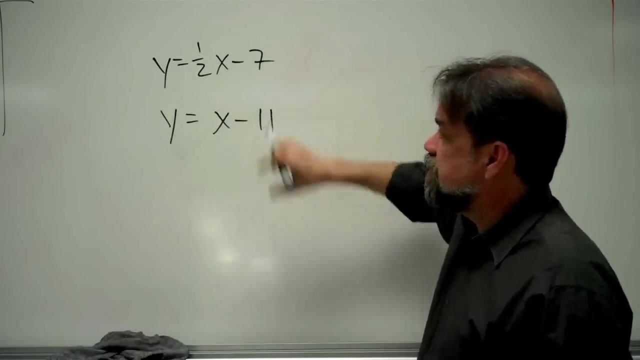 Okay, Not so hard, is it? Let's try another problem. Let's do: Y equals 1 half x minus 7 and y equals x minus 11.. Okay, We're going to do the exact same thing. We're going to say: this equation is going to equal this equation. 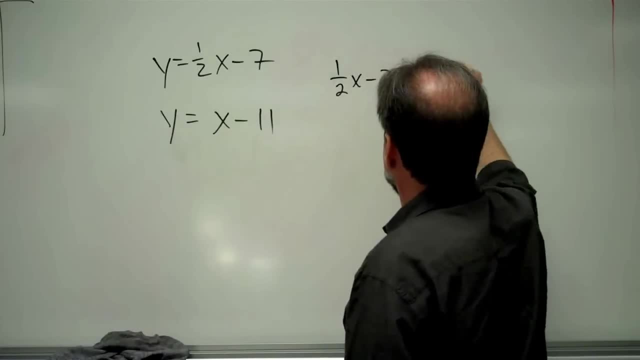 So I get 1 half x minus 7 equals x minus 11.. Again, a lot of x's up there. Let's get rid of some of them. Let's subtract: 1 half x minus 7 equals x minus 11.. 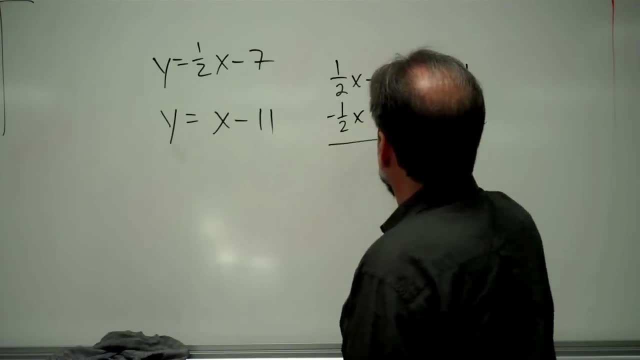 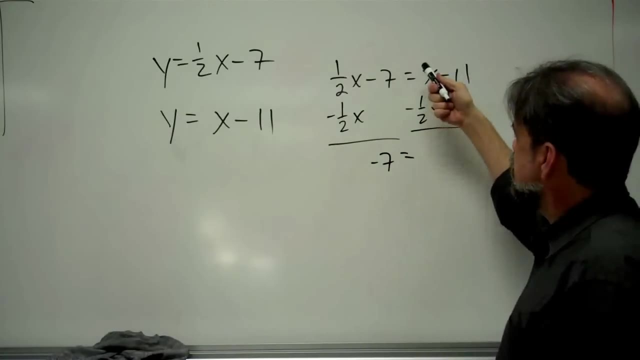 1 half x minus 7 equals x minus 11.. 1 half x from both sides- And I get These cancel out Negative 7 equals x minus half of an x. That's like saying 1 minus 1 half. 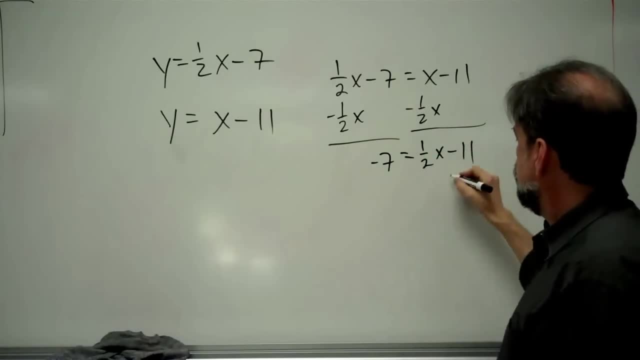 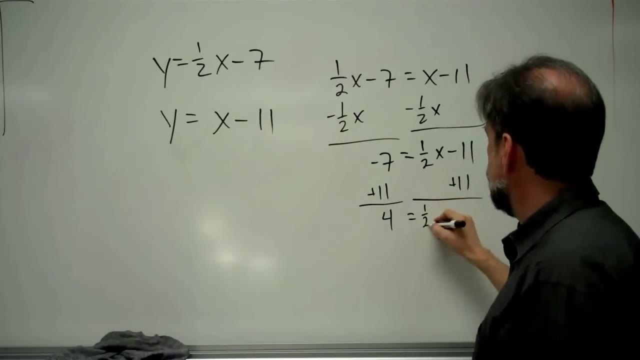 That's 1 half x minus 11.. Now I'm going to add 11 to both sides And I get negative. 7 plus 11 is 4, equals 1 half x. So 1 half of what number equals 4?? 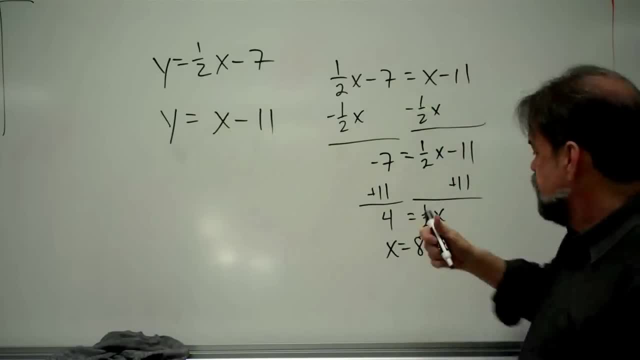 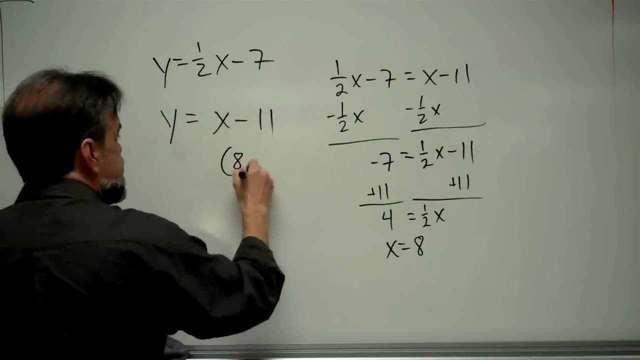 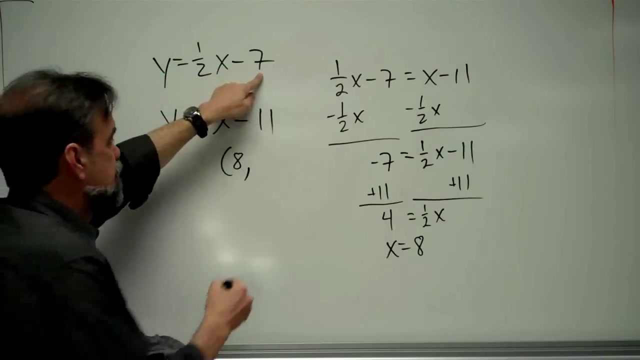 I believe x would be 8.. Okay, Dividing by 1 half is the same thing as multiplying by 2. And so I get x equals 8.. Great, That means my point is 8 something. Half of 8 is 4 minus 7 is negative 3.. 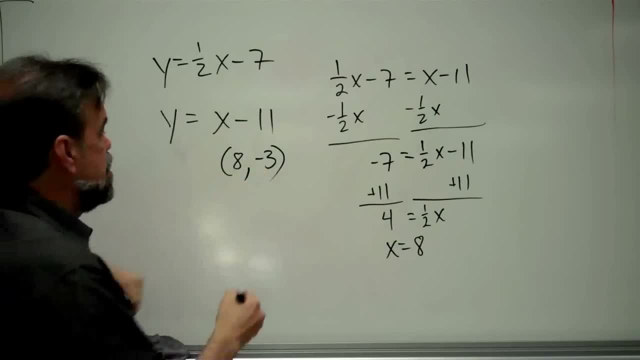 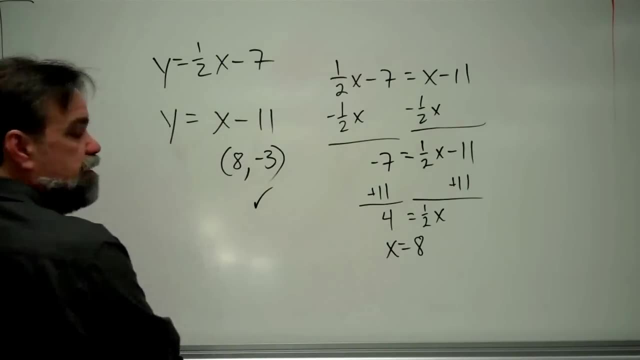 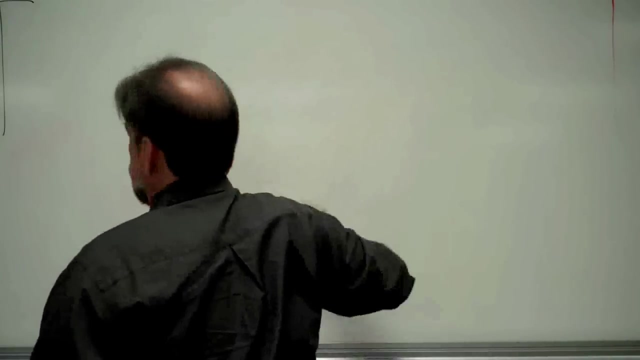 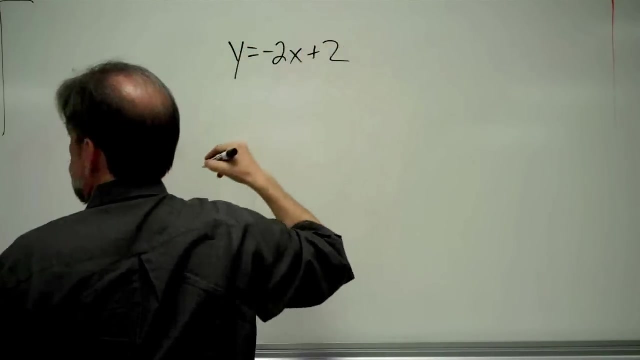 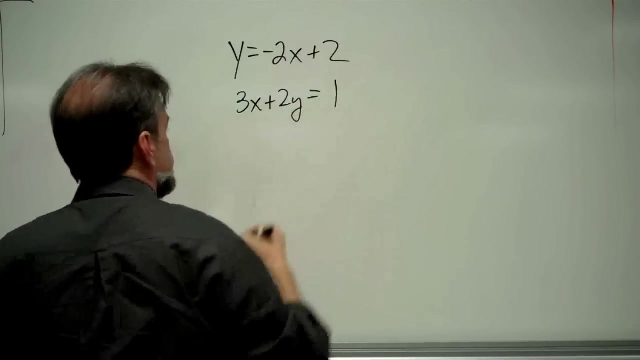 And 8 minus 11 is also negative, 3.. So, again, it works. Okay, Let me give you one more, And this one's going to have a little twist to it. This time we have: y equals negative 2x plus 2, and 3x plus 2y equals 1.. 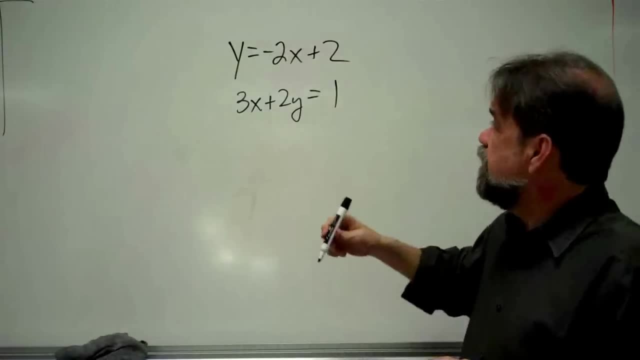 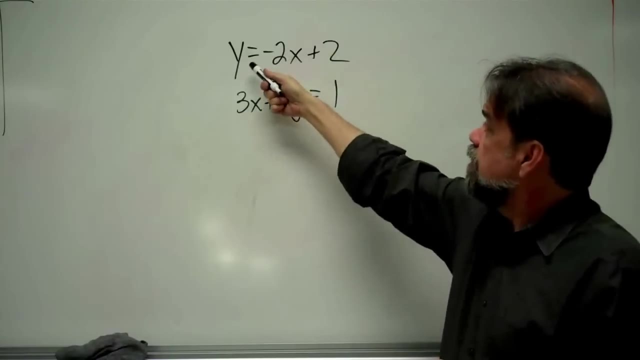 All right Now. you've already noticed what's different about this one, And that is this line right here is not written in slope-intercept form. This one is: It's solved for y. y equals mx. My slope is negative 2.. 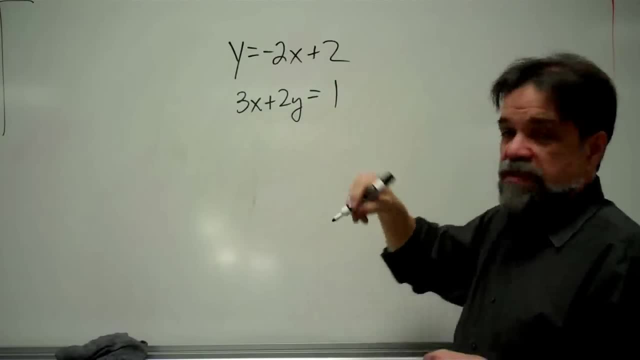 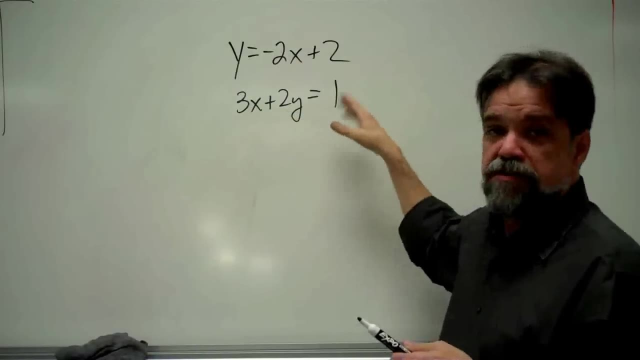 My y-intercept is the point 0, 2.. This line's not written right, though, So one option would be: you subtract 3x from both sides, You divide both sides by 2.. You solve for y. You figure out what the 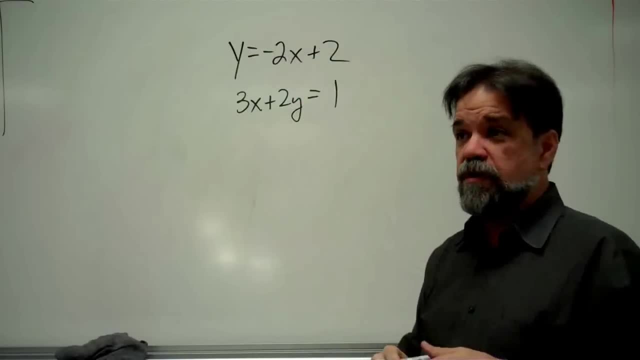 And then you set this equation equal to that equation. That's a perfectly fine way to do it. Actually, let me take that back. That's an okay way to do it. I don't recommend doing it that way. Okay, It's. 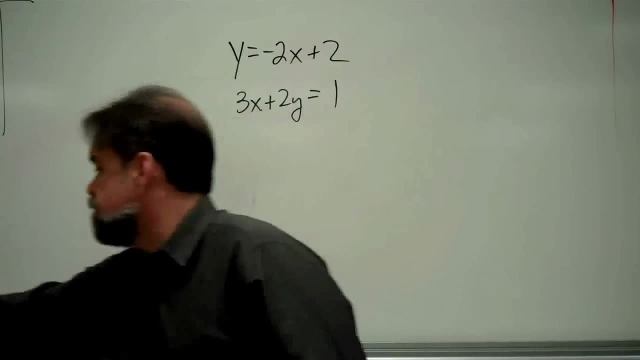 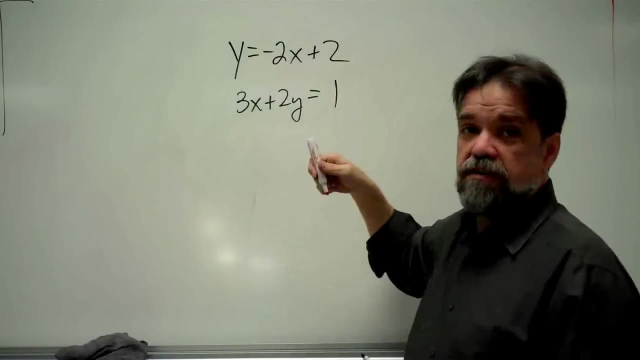 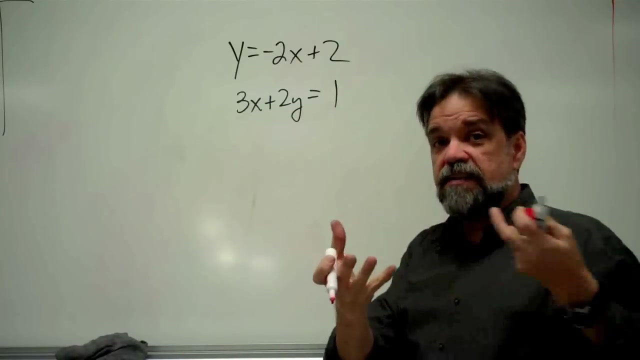 It ends up being the hard way. Let me show you a much easier way. y is negative 2x plus 2, right, y equals that. That means y and negative 2x plus 2 are exactly the same thing. And if one thing is exactly the same thing as another thing, 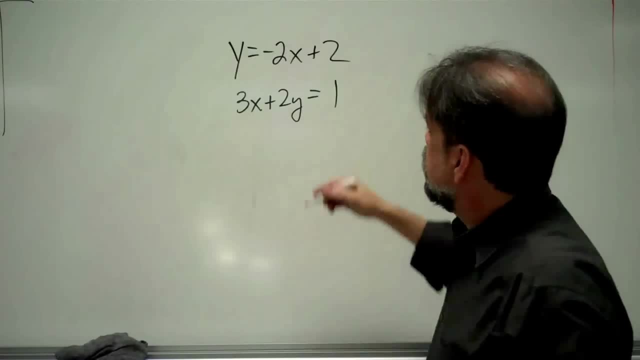 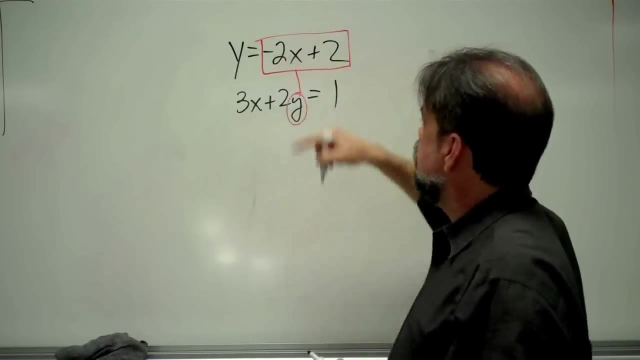 those things should be interchangeable. So what I can do is I can take this, and let me just replace this y here with negative 2x, Negative 2x plus 2, because after all, they are the same thing. All right, 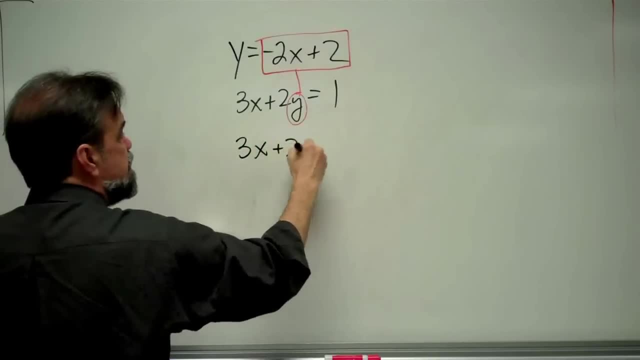 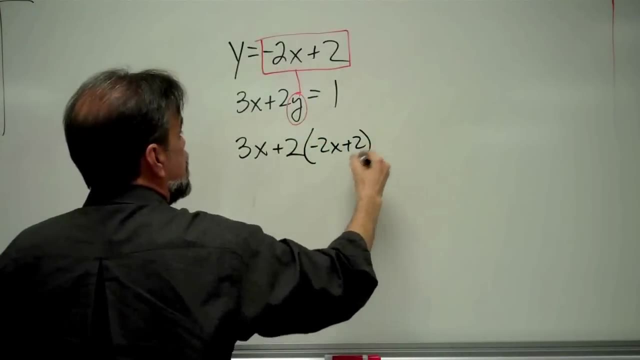 Let's just make that little substitution. We've got 3x plus 2 times, and I'm not going to call it y this time, I'm going to call it negative: 2x plus 2.. And that equals- finish it off here- 1.. 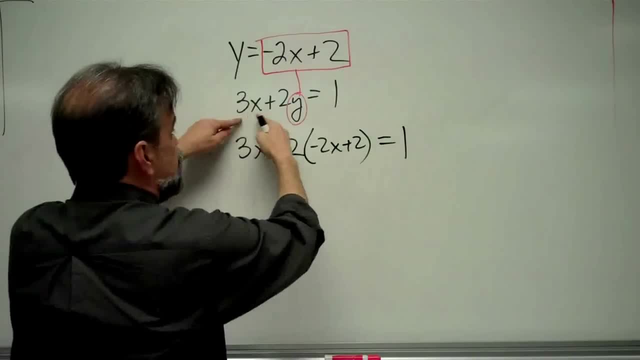 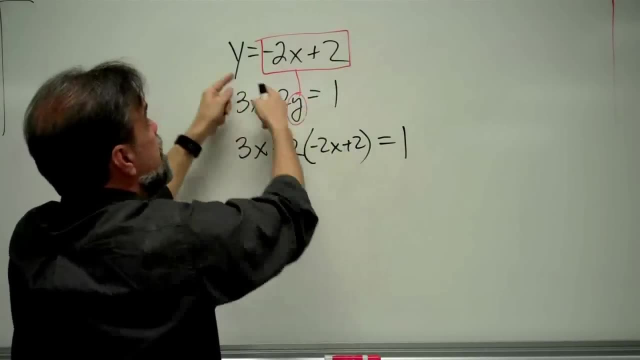 Okay, Let me show you again exactly what we're doing here. We're just rewriting this line, except instead of saying y, I'm saying negative 2x plus 2.. And why am I doing that? Because y equals negative 2x plus 2, because it's the same thing. 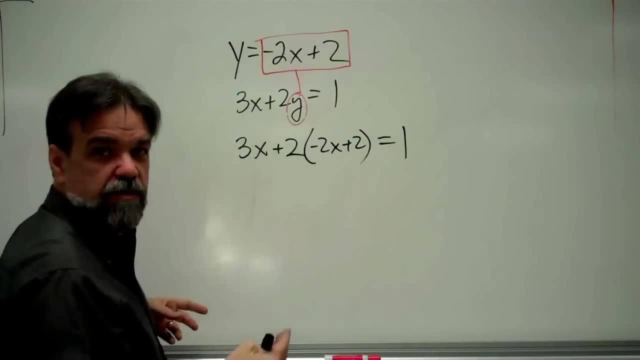 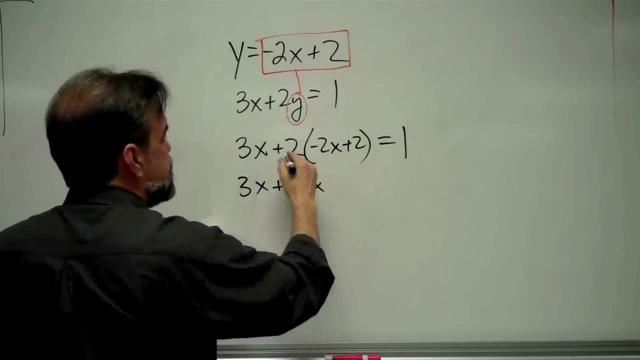 All right, We know how to solve this. Distribute, combine like terms. Let's go ahead and do it. It's pretty easy. 3x plus 2 times negative, 2x is negative. 4x 2 times 2 is 4, equals 1.. 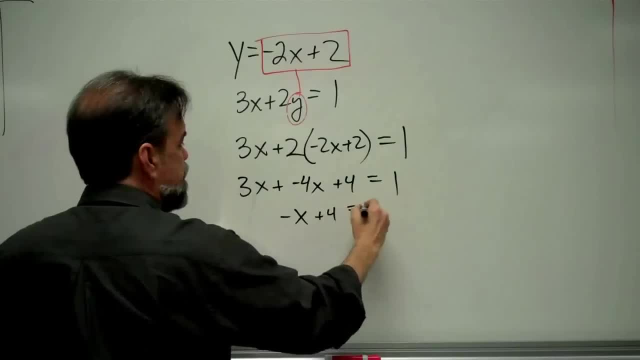 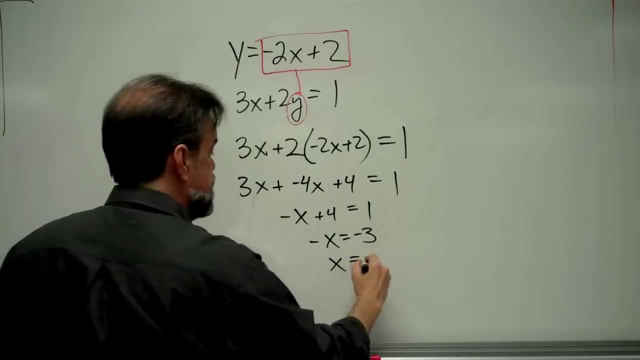 3x plus negative 4x, that gets me a negative. x plus 4, equals 1.. Subtract the 4, and I get negative. x equals negative, 3.. Multiplying times negative, 1,, I get x. I get x equals 3.. 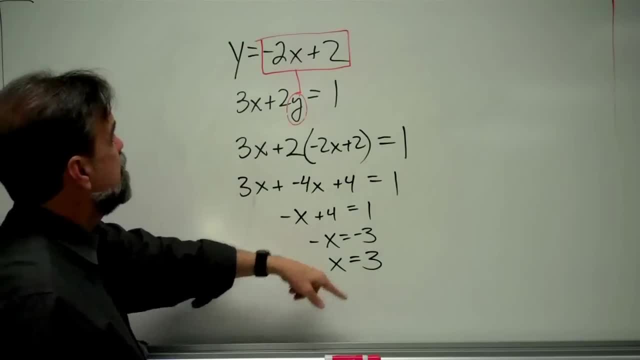 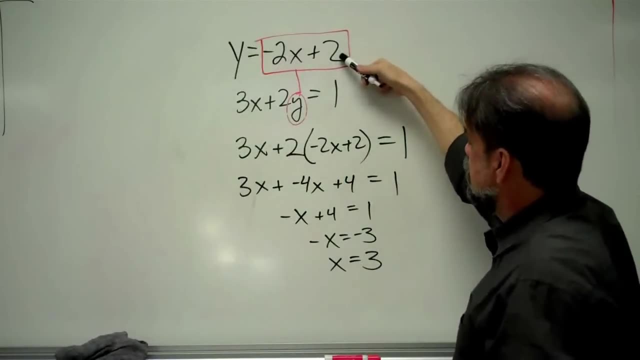 Okay, And if x is 3,- let me pop that back up here- And negative 2 times 3 would be negative 6, plus 2 is negative 4.. So it looks like my answer is 3, negative 4.. 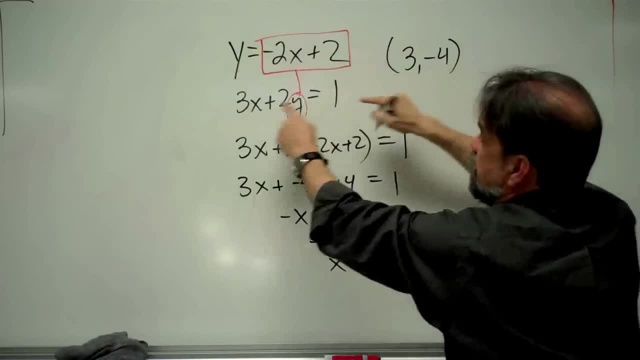 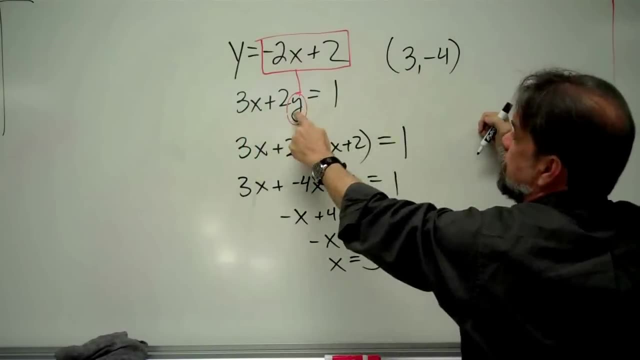 Let me just take this point, which I know works for this one, and see if it works for this line: 3 times 3 is 9, plus 2 times negative, 4 is negative 4.. So I get x equals 3.. 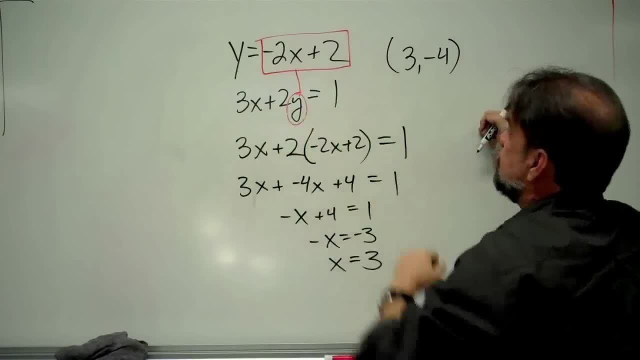 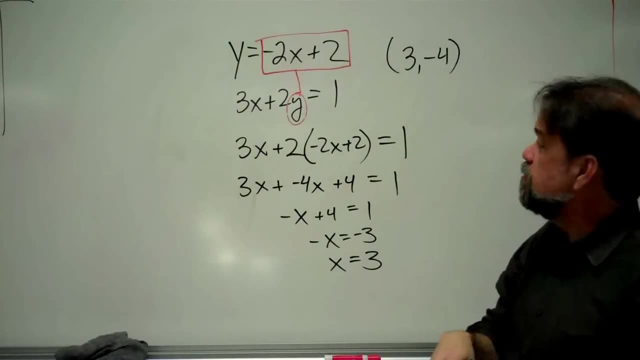 Negative 8, and 9 plus negative 8 does equal 1.. So this point is on this line and it's also on this line, and that means it's the intersection point. Okay, This method here- actually the method we've been using this entire time- is called the. 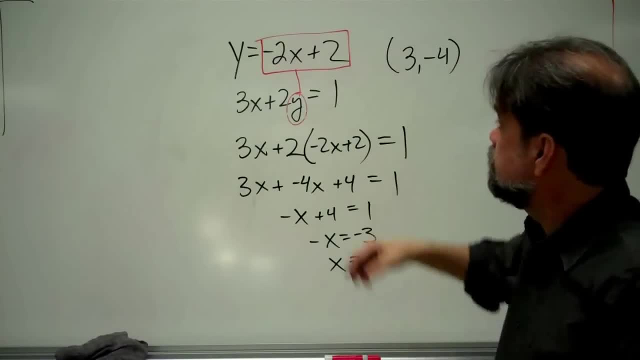 substitution method, and the reason it's the substitution method is we're taking what y equals and we're substituting y for that expression instead.